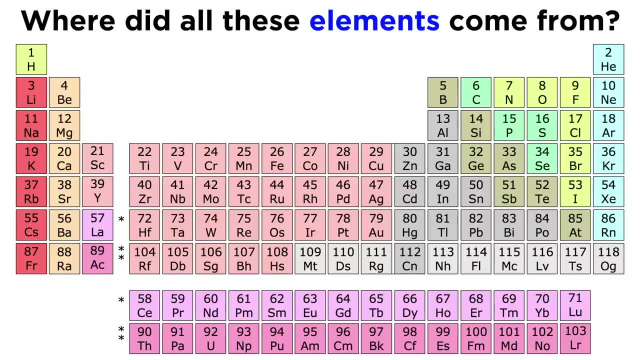 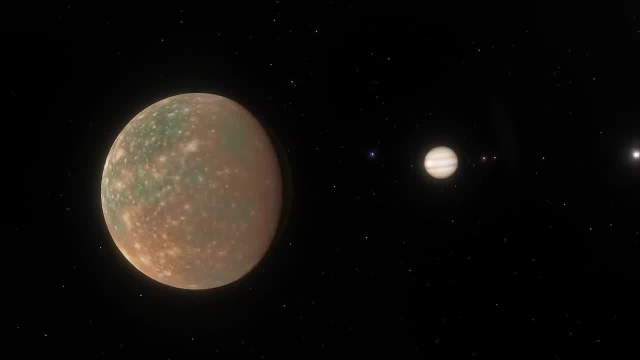 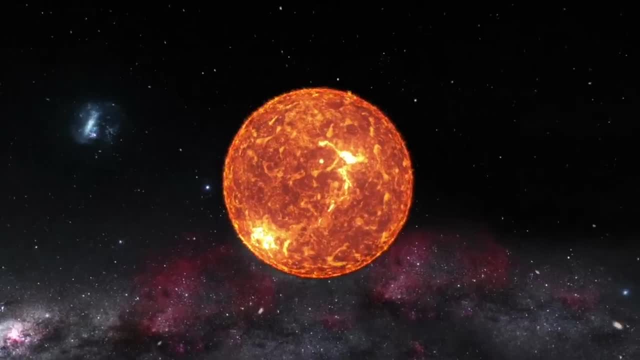 But we still haven't talked about all the other elements on the periodic table. We've only mentioned hydrogen and helium so far. So where did the rest come from? And what about all the planets and moons? how did those get here? The answer to all of these questions will make sense once we learn more about what goes. 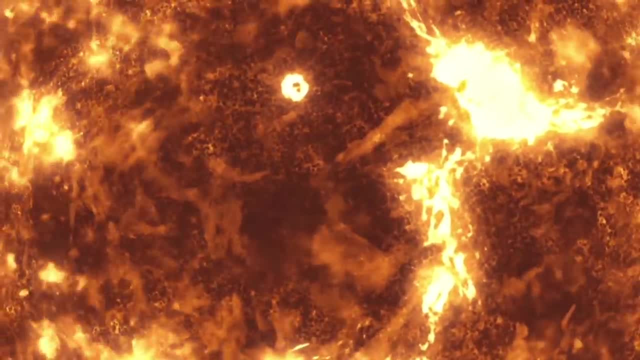 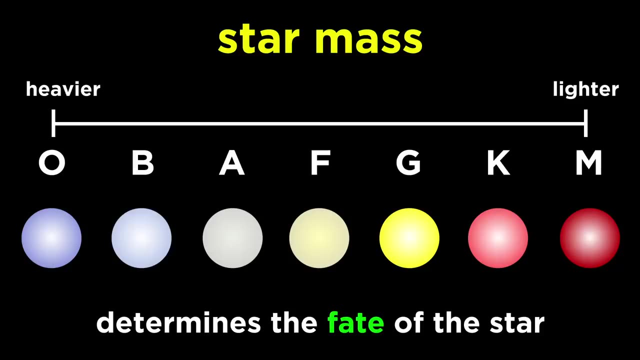 on inside a star from the moment they are born to the time of their death. That's right. stars actually die, so to speak, And the type of death, along with what's left over, will be one of a variety of possibilities. 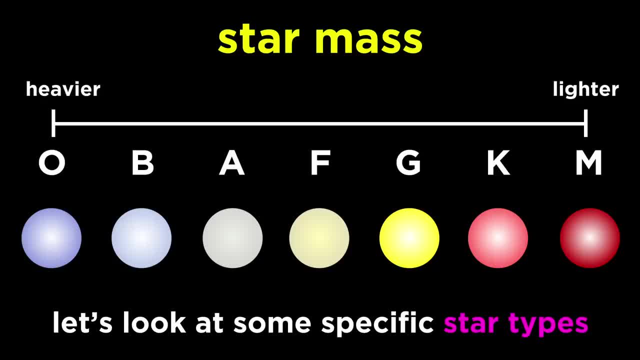 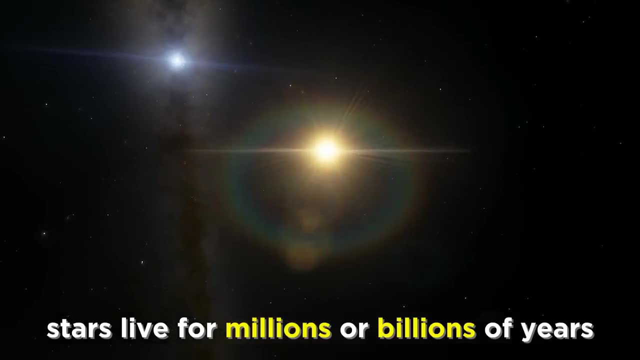 depending entirely on what happens. So let's go through the lifetime of a few different kinds of stars so that we are ready to understand the next 13 billion years of development in the universe. The life cycle of any star, from birth to death and all the stages in between, will. 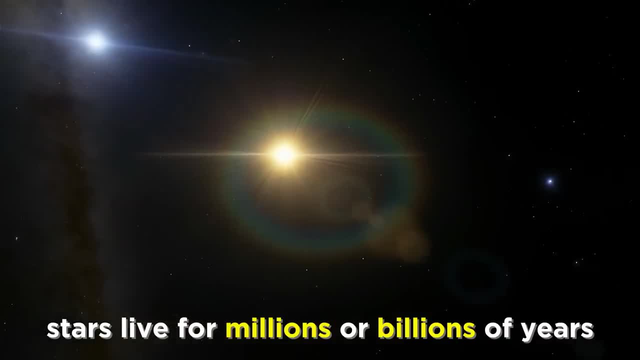 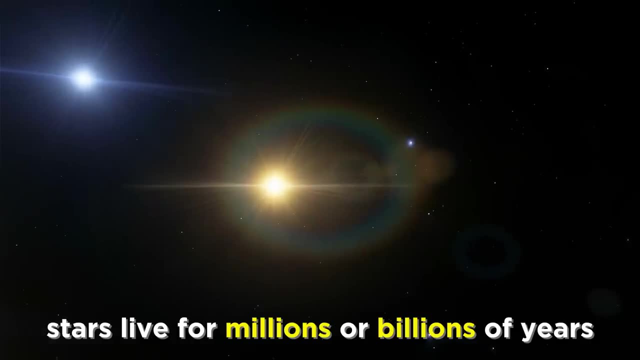 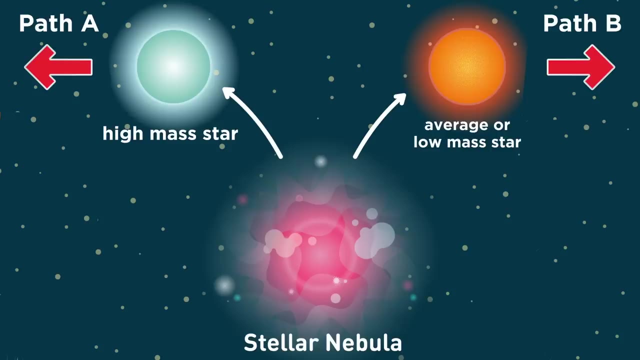 span millions or even billions of years. This is why stars don't seem to change at all, because a human lifetime is a snippet of a fraction of a blink of an eye to these behemoths. The path that will be followed by a particular star depends mainly on its mass, or how much. 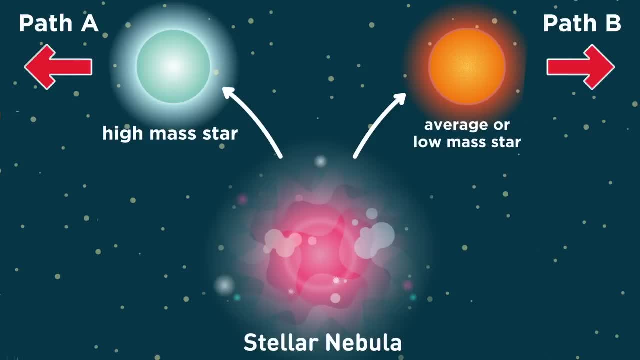 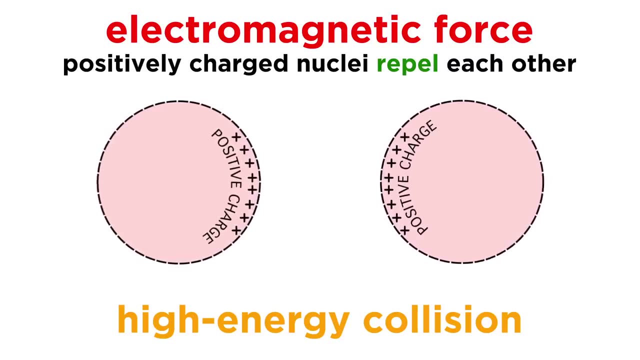 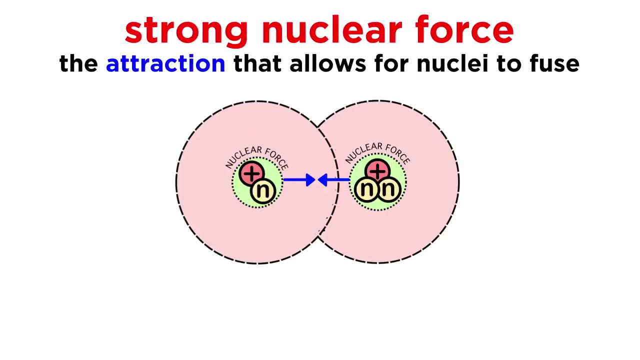 gas collected and collapsed to form the star, because that material will serve as the star's fuel. As we may remember from physics and chemistry, when nuclei collide with enough energy so as to overcome the electromagnetic repulsion between them, the strong nuclear force takes. 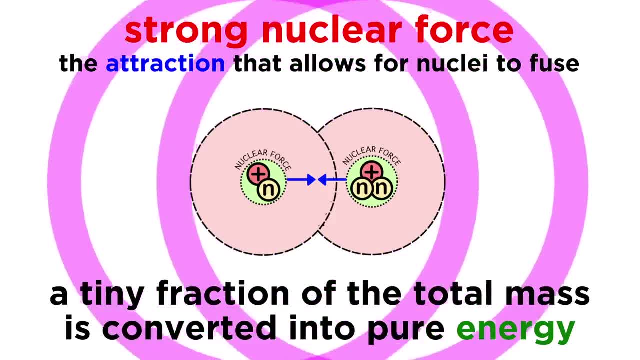 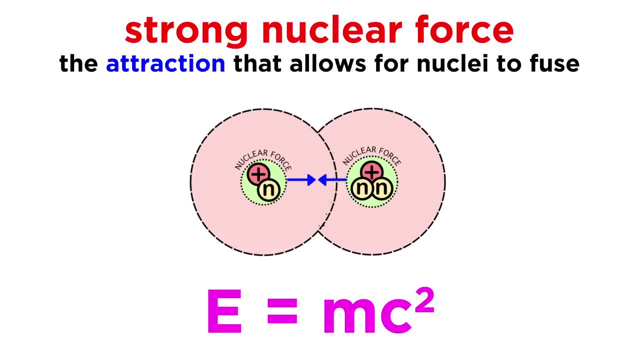 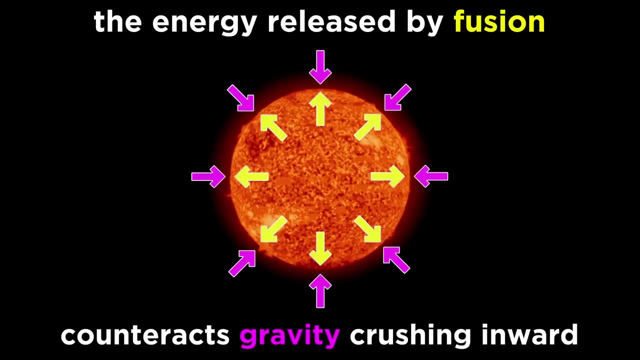 over and they fuse, with a small fraction of their mass converging on the other side. This is what happens when a star is converted into huge amounts of pure energy, as dictated by E equals mc squared. Therefore, only by colliding nuclei together and fusing them in its ultra-hot core can 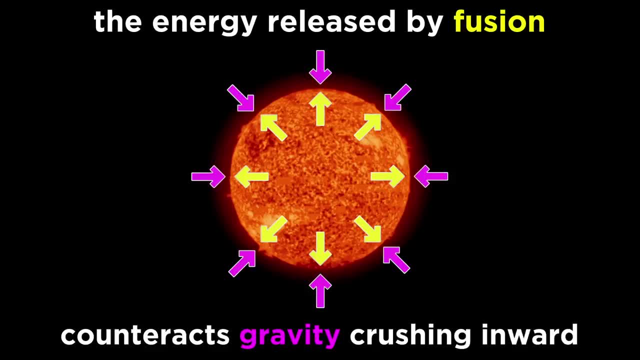 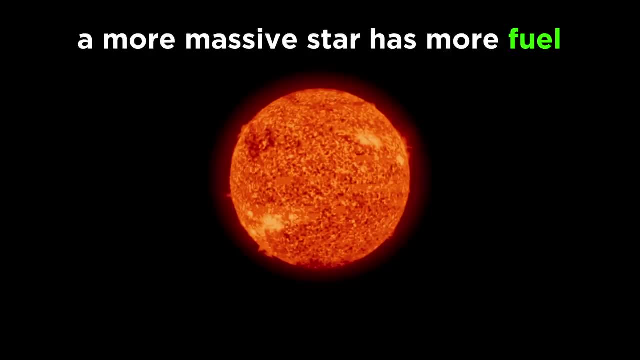 a star release enough outward energy to counter the effects of gravity relentlessly crushing inward. This means that the amount of matter that forms the star determines the amount of fuel and, through a variety of other factors, the lifetime and efficiency of the star's energy will be determined. 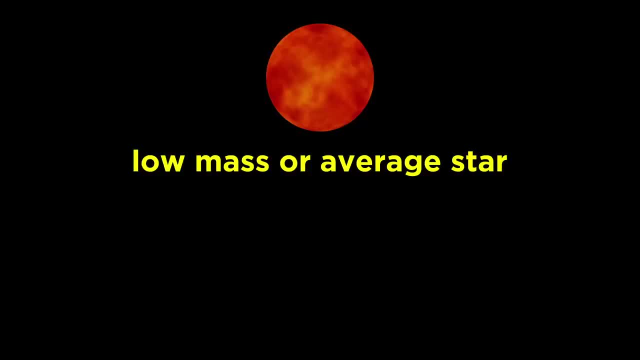 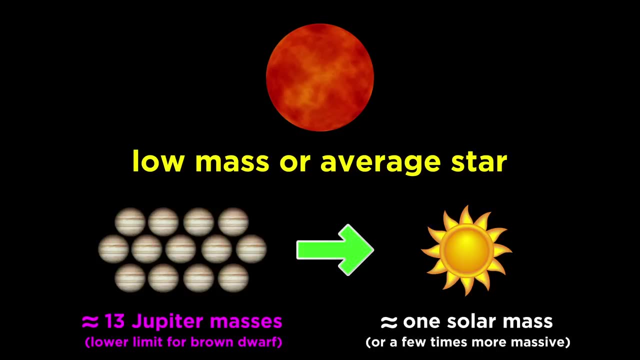 And thus the star's mass will be determined as well, Given that mass is the key factor here. let's start with a low-mass star. This would range from the smallest that stars can be, meaning the smallest amount of material that can sufficiently trigger nuclear fusion so as to qualify as a star, which is about 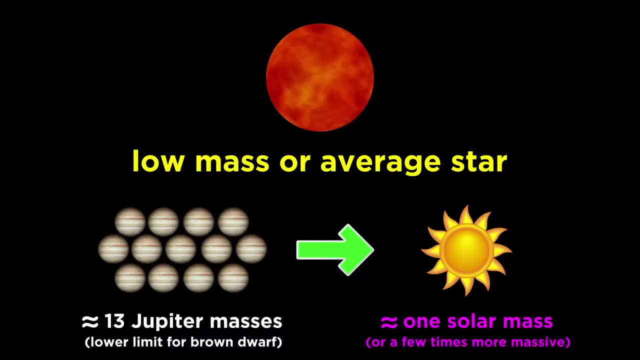 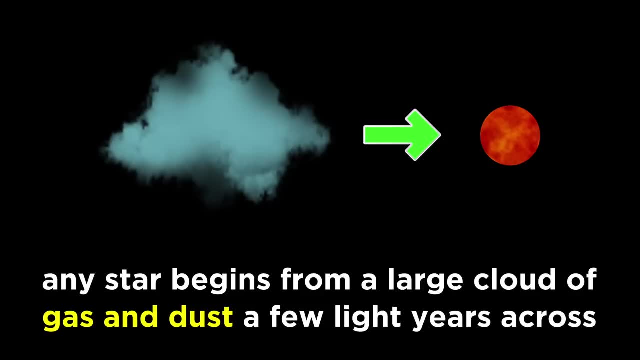 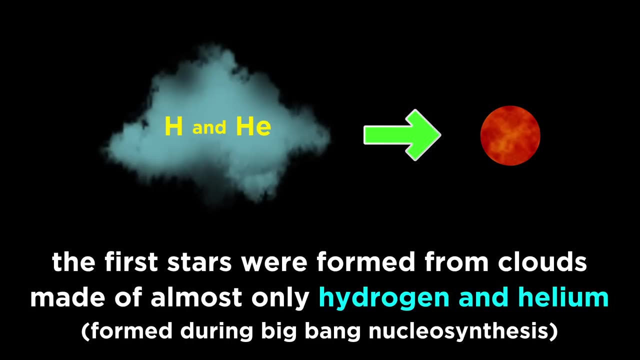 13 Jupiter masses to a star somewhere in the ballpark of our sun's mass. As we already know, any star is a mass. any star will begin as a cloud of gas and dust at least a few light years across. In the earliest era of star formation, this material was almost exclusively hydrogen and 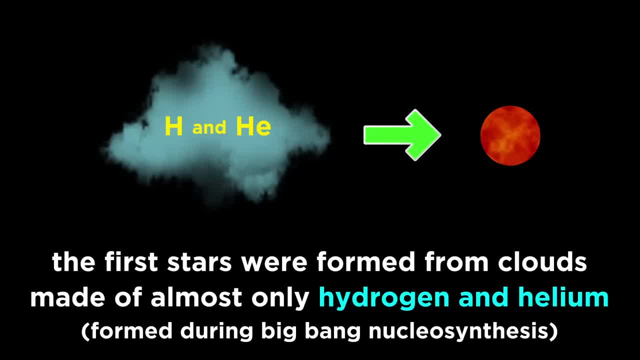 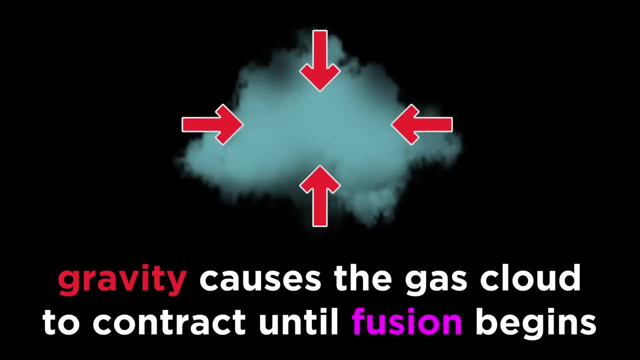 helium, as this was what remained after the brief 17 minutes of nucleosynthesis soon after the Big Bang. This matter collects due to gravity pushing increasingly inward as it contracts, until things get so hot, over a few million years, that nuclear fusion eventually begins establishing. 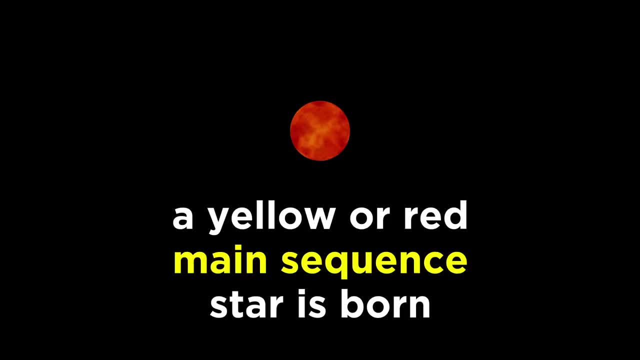 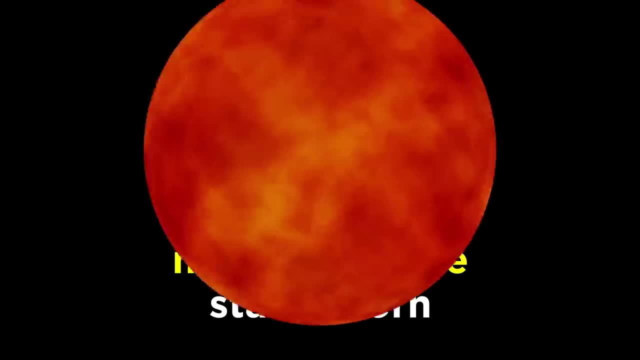 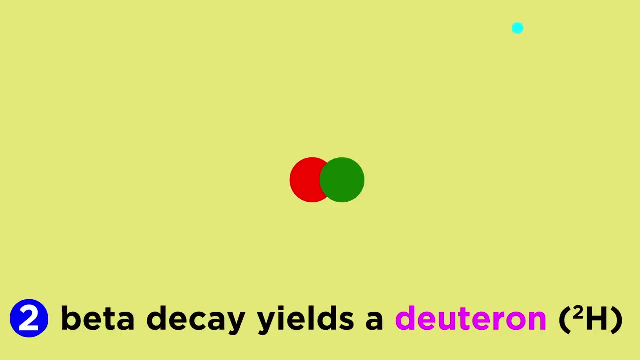 an equilibrium and generating a yellow or red main sequence star that glows with all the energy released from the collisions happening inside. These fusion reactions begin with two protons fusing, followed by subsequent beta decay to get a proton and a neutron, and we call this a deuteron. 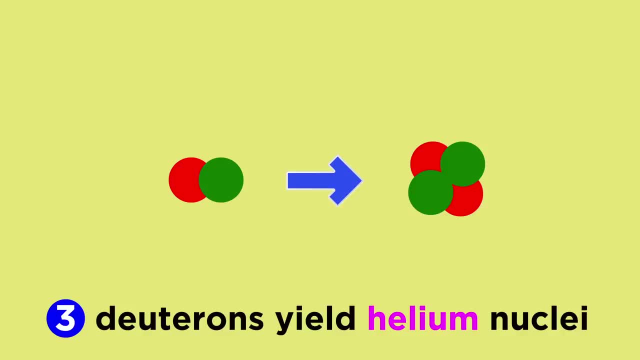 Deuteron, which is a nucleus of heavy hydrogen. Then deuterons are involved in reactions that make helium, which has two protons and two neutrons. Such a star will continue in this manner for billions of years, slowly fusing all of the 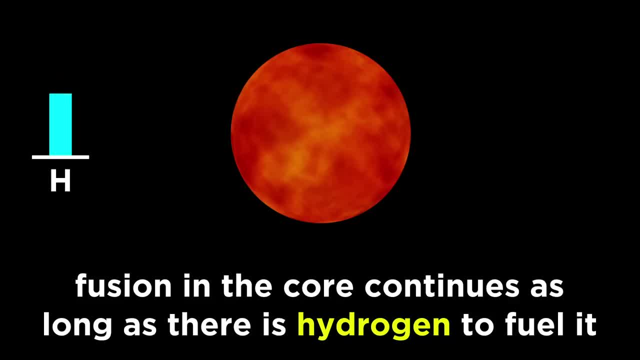 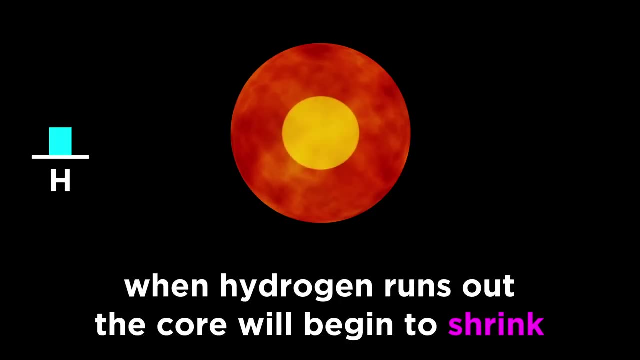 hydrogen in its core into helium and maintaining a relatively steady size, temperature and luminosity, as it does so, until almost all of the hydrogen is gone. At this point things really begin to change. The core of the star will shrink and get hotter, which makes the remaining hydrogen burn even. 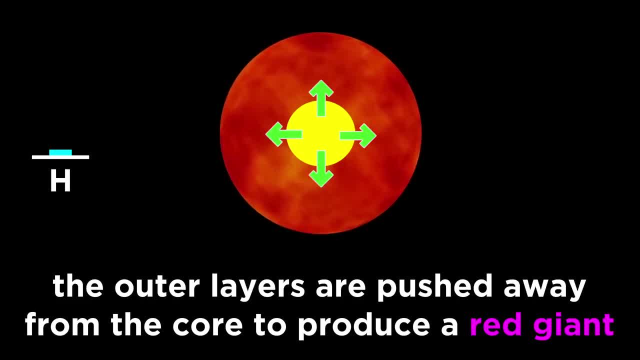 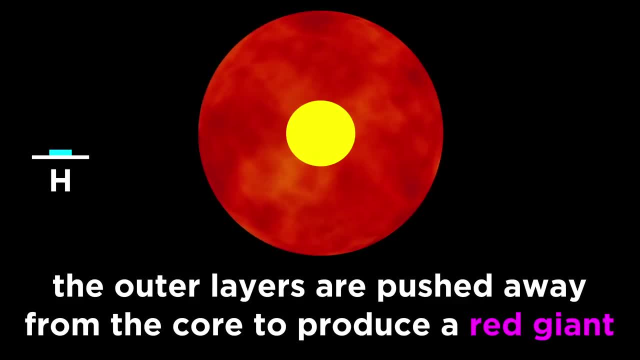 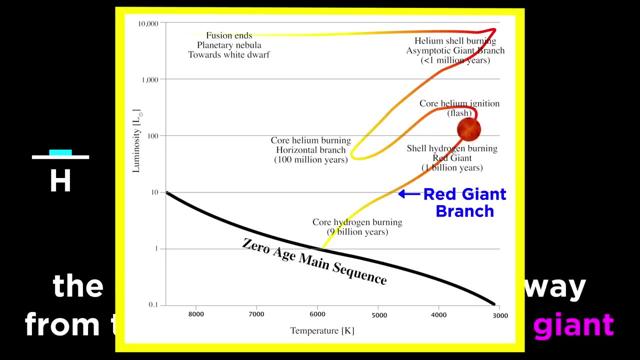 faster, and all of that extra energy being generated will radiate outwards and push the outer layers away from the core. As the outer layers expand, they cool and thus become more and more red and the star climbs up the red giant branch until we have a red giant star. 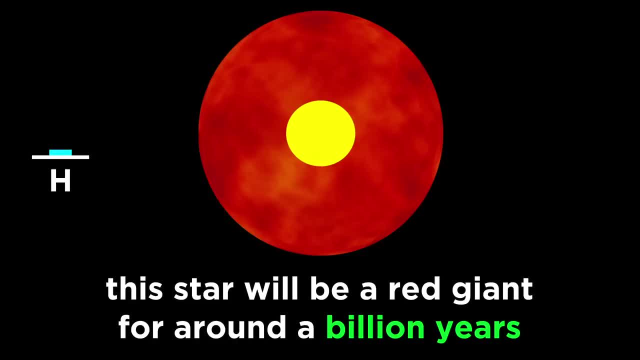 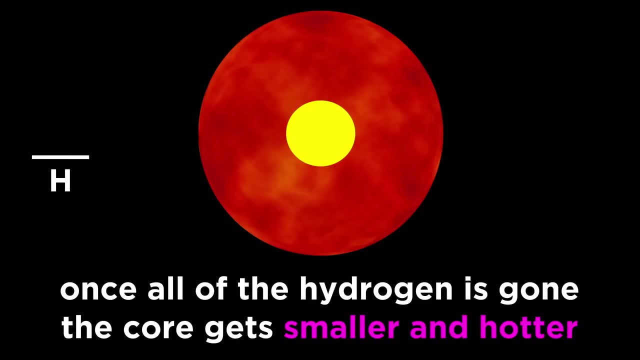 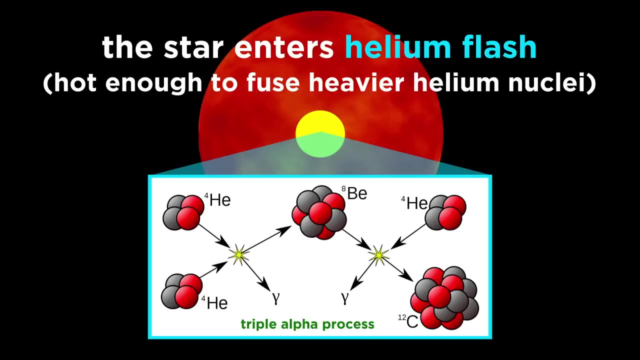 The star can maintain this new status for a little while longer, around a billion years. but after almost all the hydrogen is gone, the core gets even smaller and even hotter. At this stage, a phase called helium flash- Things are so hot that the star is able to fuse these heavier helium nuclei into larger 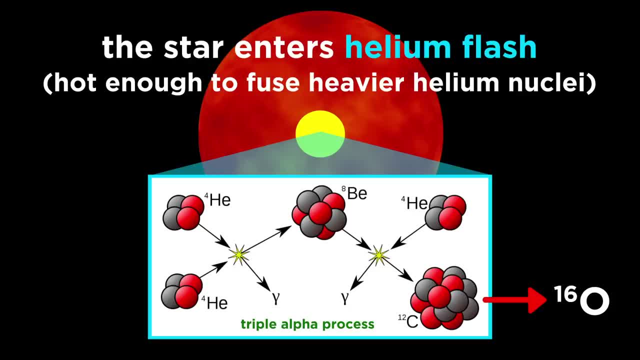 nuclei like carbon, and then oxygen through something called the triple alpha process. This process is called the triple alpha process, And this means that the star has a whole new source of fuel in all the helium it has been making for billions of years. 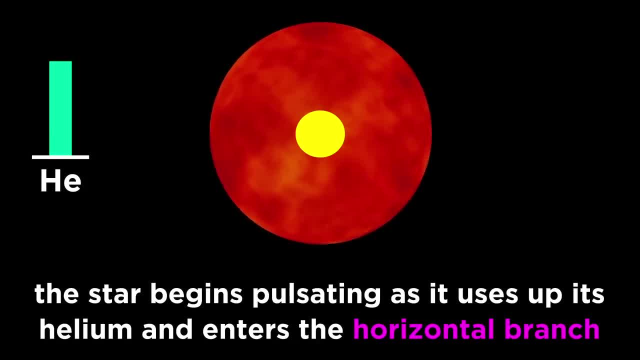 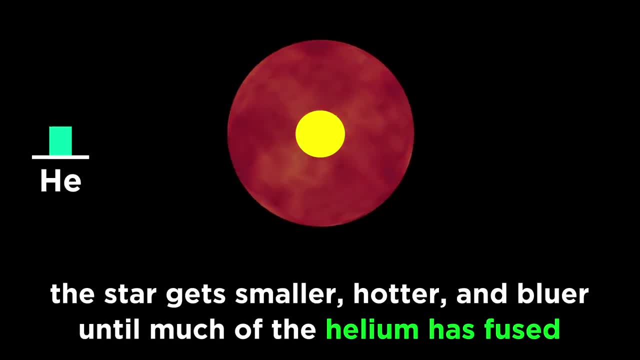 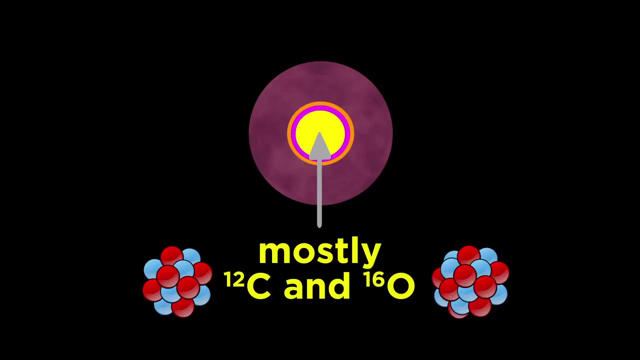 The star begins pulsating as it runs through its final energy reserve, entering what we call the horizontal branch, and in this time it becomes smaller, hotter and bluer until, at last, much of the helium has been fused into larger nuclei. Once the core is predominantly carbon-fused, the core will become more and more red and 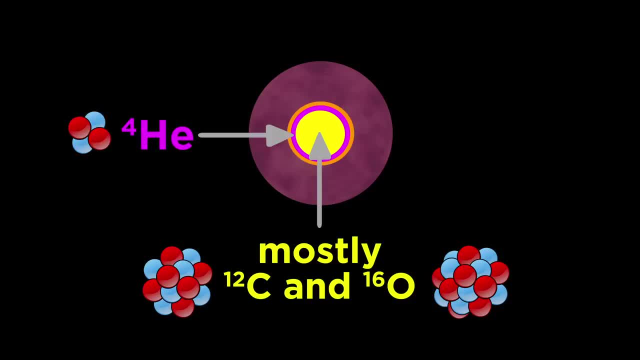 hotter. When the core is predominantly carbon and oxygen, with just a shell of helium around it and a shell of hydrogen around that, the star has very little material left to burn, so the core will collapse and the star enters the asymptotic giant branch. This means it will grow rapidly and become a giant star again, until the last bursts of energy eject the outer layer, pushing it away from the core and back into the interstellar medium, leaving only a tiny, very hot, bare core behind, about the size of Earth. 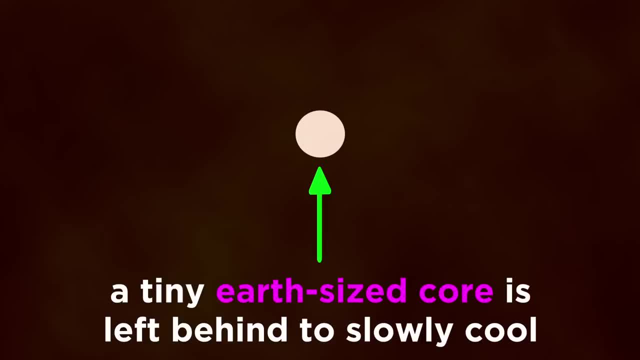 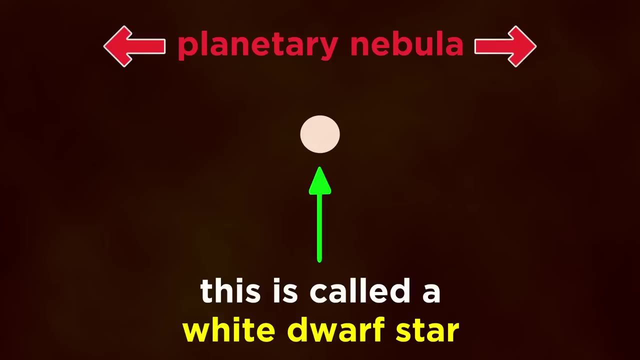 This will gradually cool as it has no more fuel to burn, not being hot enough to fuse carbon or oxygen nuclei, and it will contract further until we are left with a white dwarf star. The ejected shell is called a planetary nebula, which is misleading since it is not a planet. 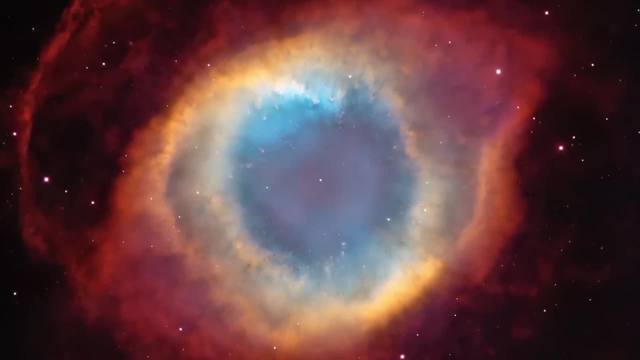 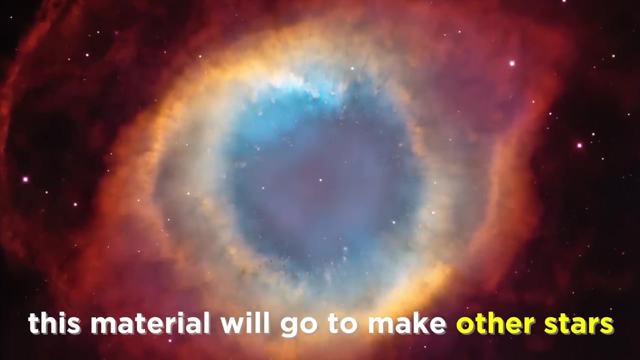 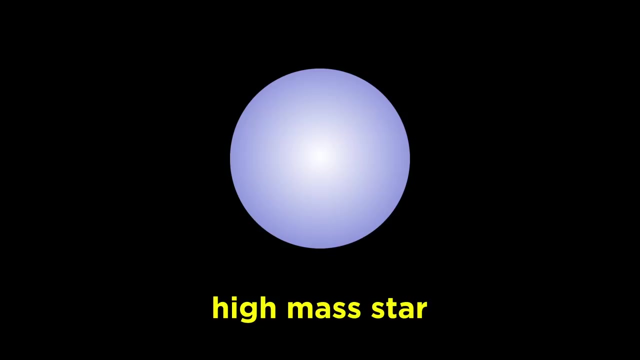 and did not come from a planet, But the name originated from the word nebula. The name originated from confusion upon its discovery and it stuck. The material in a planetary nebula will then become available to join more gas particles to form yet another star. 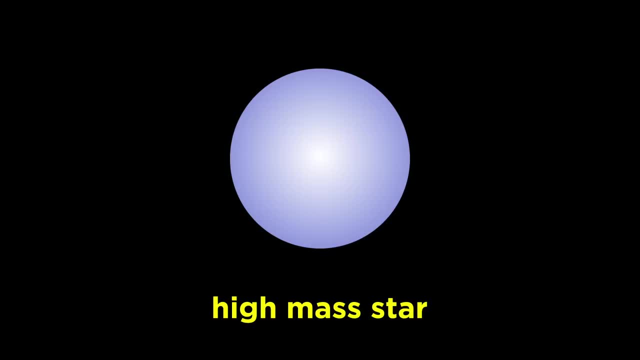 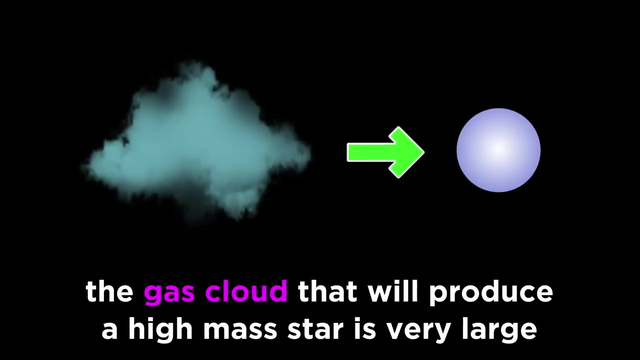 Now for a high mass star, one's much more massive than our sun, things are quite different. Their demise will not be so quiet. Big stars go out with a bang. Things start out normally with a gas cloud under the influence of gravity. It is simply that this cloud will be much. 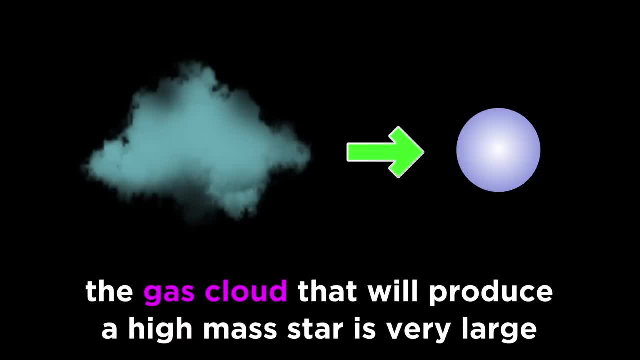 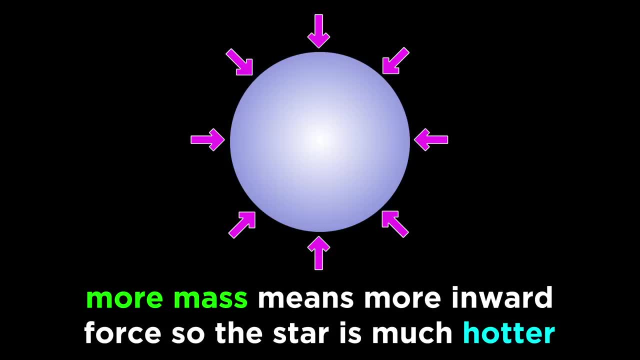 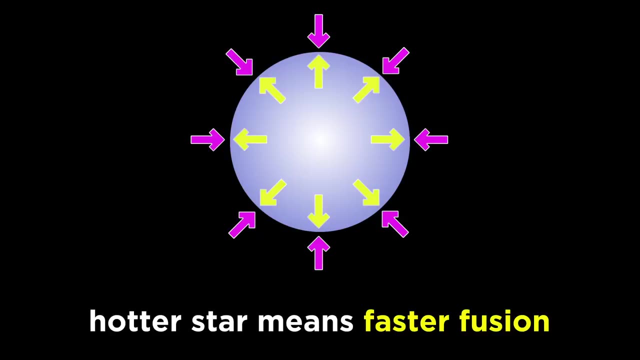 larger than those that form low-mass stars, so it will contain much more mass. More mass means more gravity, which means the force pushing inward is much stronger and the star gets much hotter. A hotter temperature means faster fusion, which generates greater outward pressure to counteract the greater inward pull of. 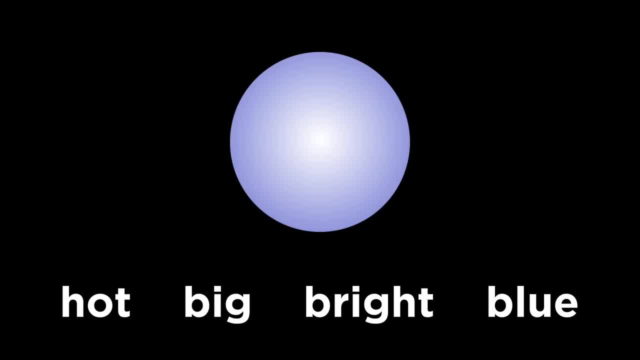 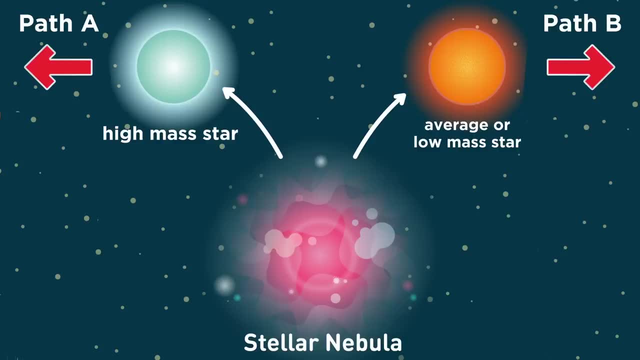 gravity. This will result in a main-sequence star that is hot, big, bright and blue. This is where things start to go differently from low-mass stars. Whereas low-mass stars take billions of years to use up all their fuel, high-mass stars are much hotter and burn their fuel much faster. That means 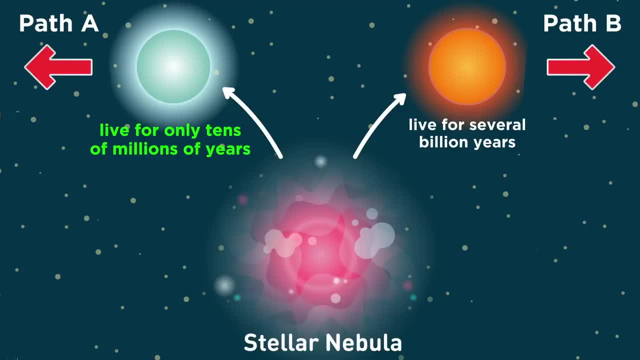 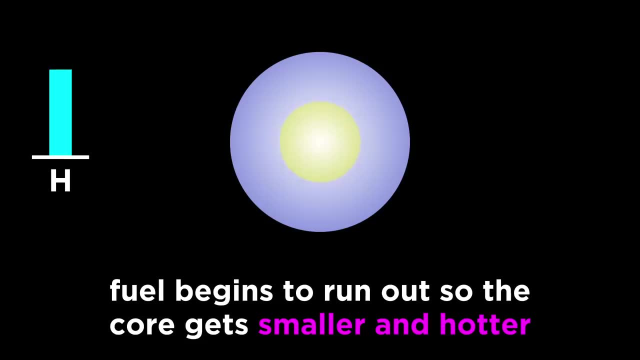 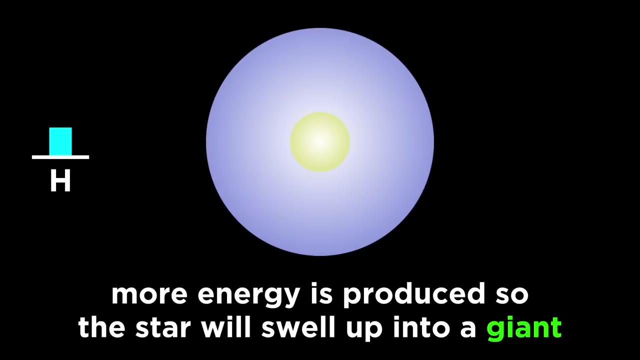 they use up all the hydrogen in their cores in around just a fleeting hundred million years, or even ten million if big enough. As the fuel starts running out, the core contracts and heats, producing more energy, so the star will swell up into a giant star, just like we saw for low-mass. 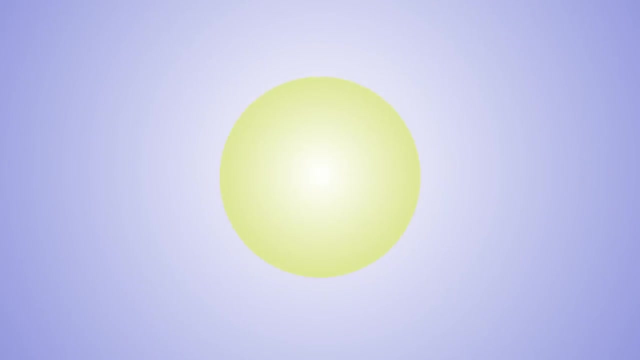 stars. But while the core of a high-mass star continues to compress, it gets much hotter than the core of a low-mass star and it becomes able to fuse helium nuclei to form carbon and then oxygen, and then neon and then silicon each. 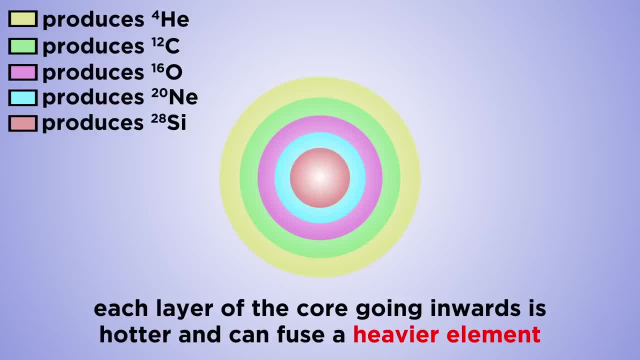 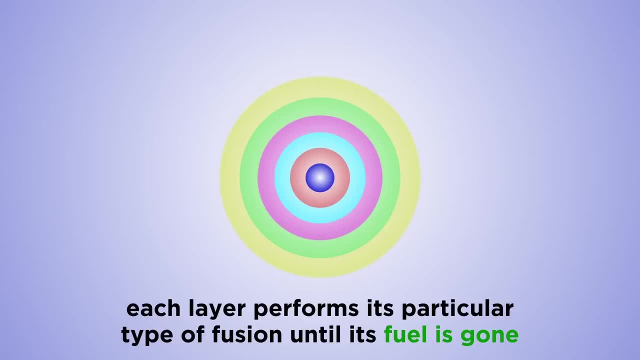 heavier nucleus that forms a giant star All the way. at the center sits the heaviest element that can be fused within a star: iron. As this occurs in these different layers, each performing a particular type of fusion until no fuel remains, the star is left with a core of 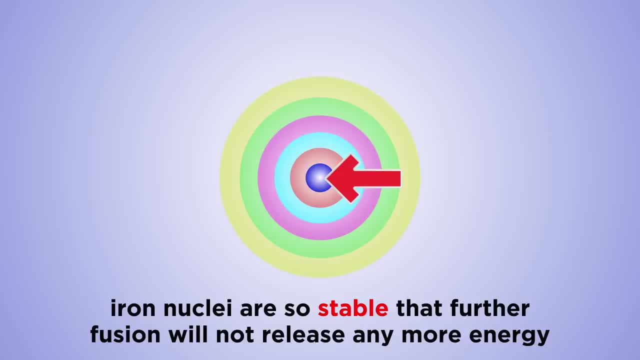 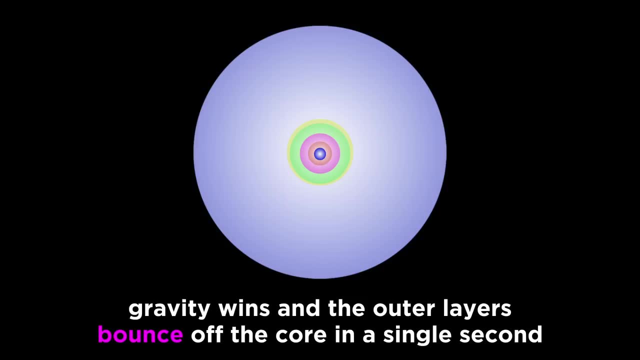 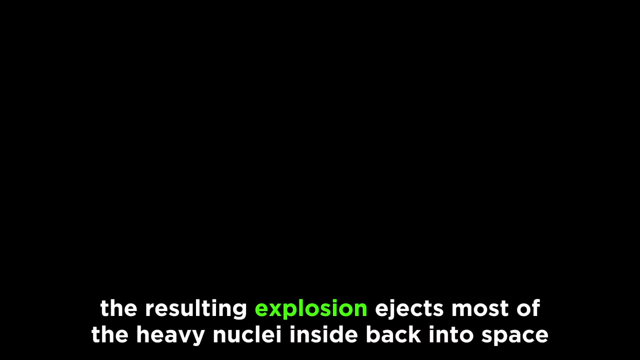 iron nuclei that are so stable that further fusion can release no more energy. At this point, gravity wins the fight and the star collapses within a single second, the outer layers bouncing off the core and triggering an explosion, thus ejecting all of the heavy nuclei, the star. 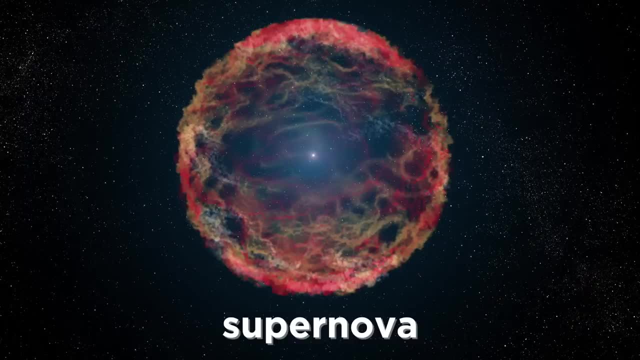 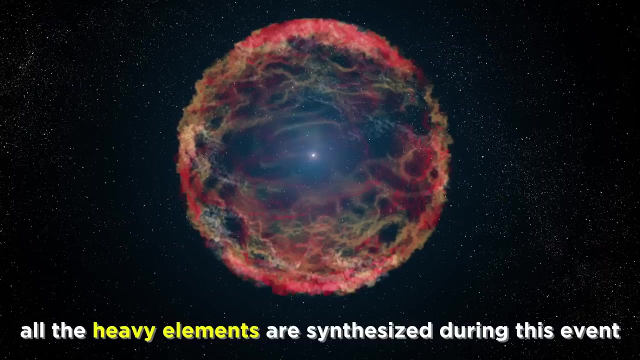 has created out into space This awesome event. one of the most violent and energetic phenomena in the universe is called a supernova. A supernova generates such an unbelievable burst of energy that, in this brief moment, Dozens of elements heavier than iron can also be synthesized. 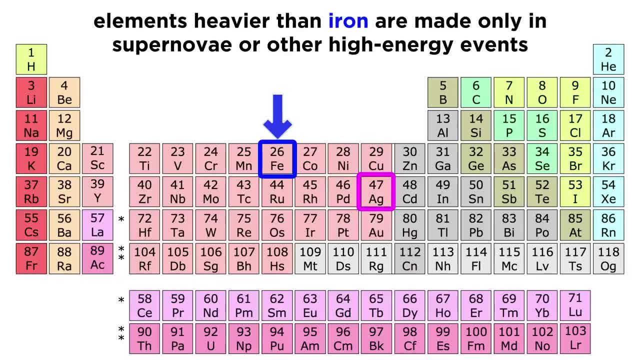 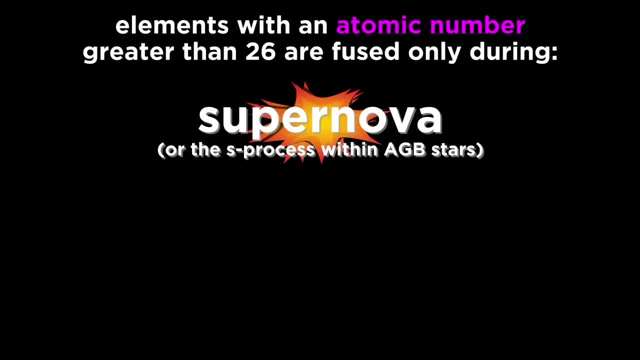 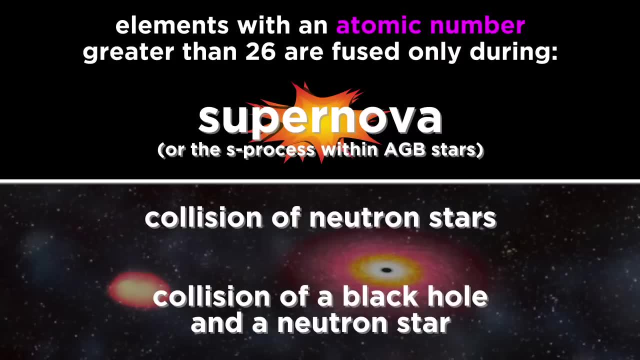 Nickel, copper, zinc, silver, gold. any element with an atomic number greater than 26 is made either in a supernova or a rare event like the collision of two neutron stars or a neutron star and a black hole, which are objects we will discuss in a moment. 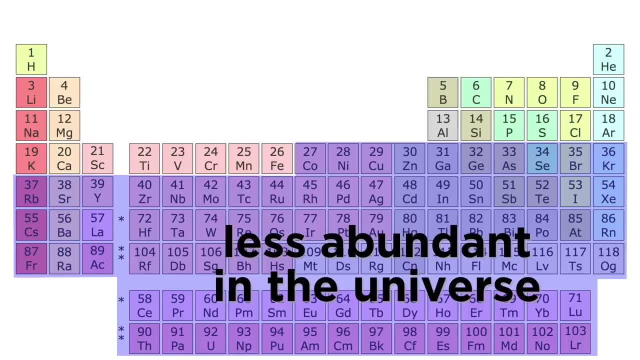 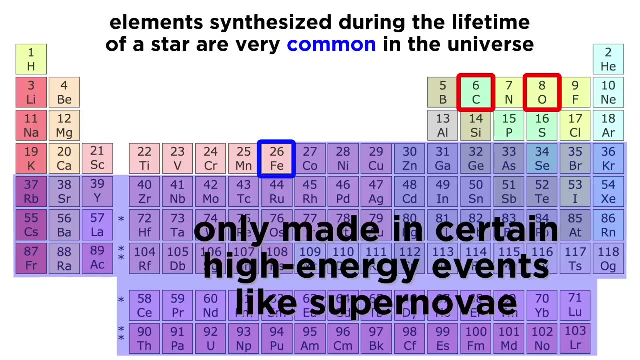 That's why these heavy elements are so rare compared to elements like carbon and oxygen, because stars can't synthesize them the way they can synthesize all the elements up to iron throughout their long lives. Nature only makes these rare elements during the death of a high mass star or in certain 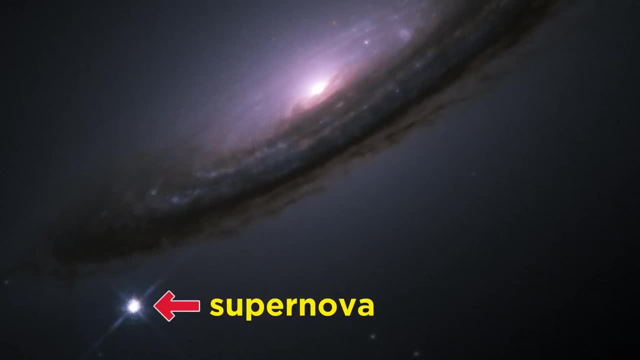 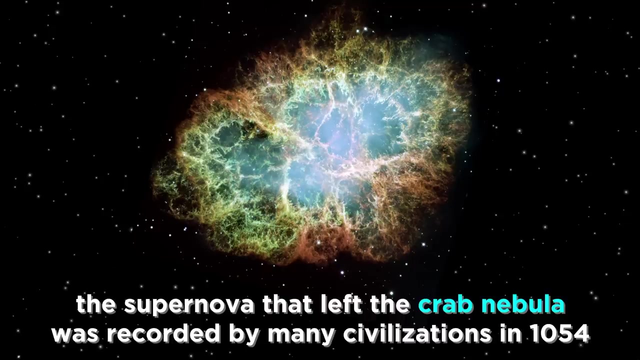 exotic collision events. Supernovae are also so bright that they are brighter than the entire galaxy they belong to when viewed through telescopes and if, in our own galaxy, they can even be visible with the naked eye, like the one that generated the famous Crab Nebula, which was 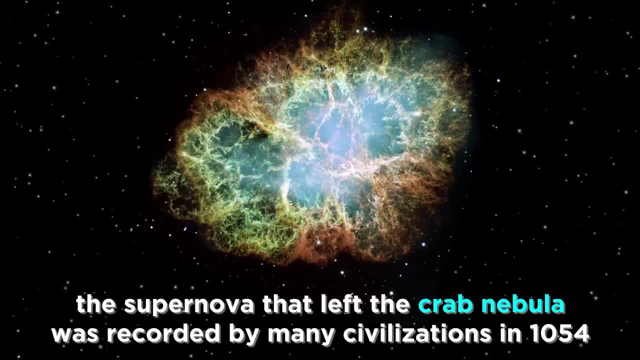 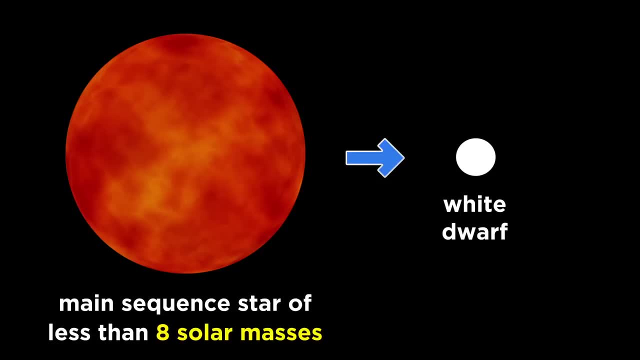 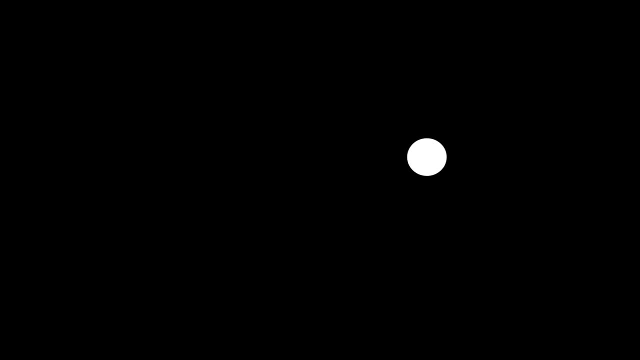 recorded by a variety of civilizations in 1054.. Now, a supernova does not leave behind a white dwarf. Lower mass stars that begin with less than about eight solar masses leave behind white dwarfs Because once reduced to zero, they become a white dwarf. 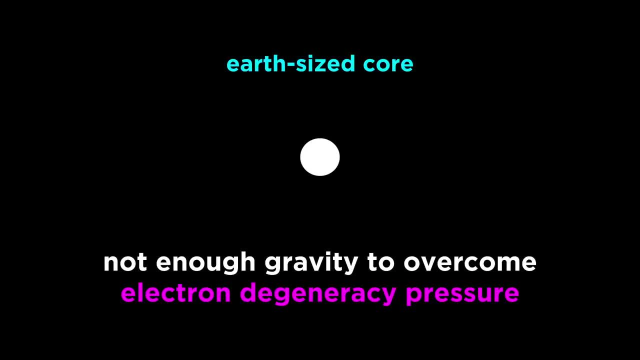 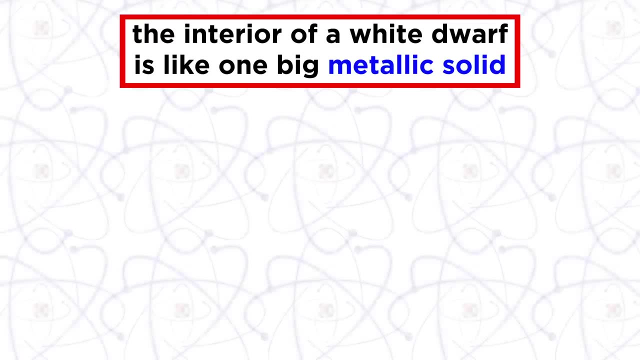 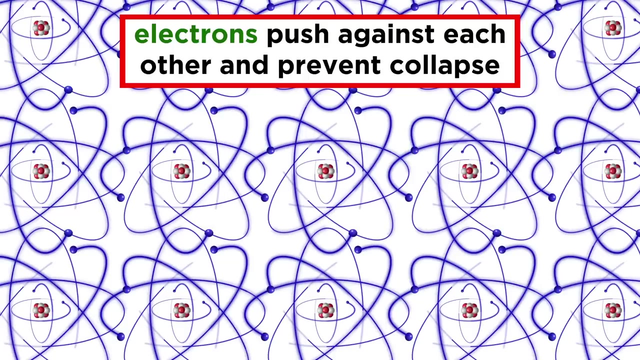 Once reduced to its lighter earth-sized core, there is not enough gravity to overcome electron degeneracy pressure. In other words, a white dwarf will become kind of like one gigantic metallic solid, with the electron clouds around the nuclei pushing against each other and preventing 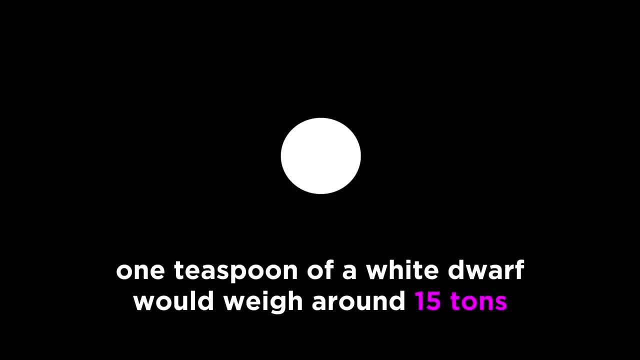 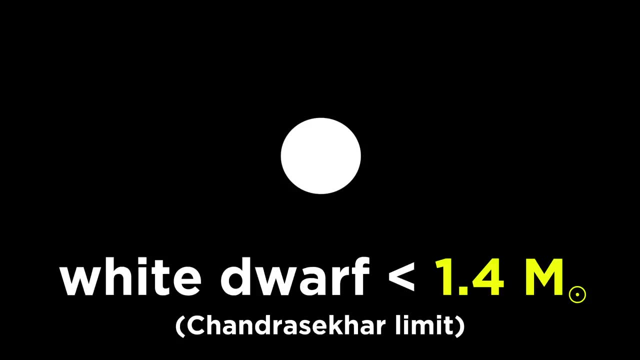 further collapse. Even still, this object is very dense, with one teaspoon weighing around fifteen tons. So below around 1.4 solar masses, the maximum mass of a white dwarf, which is also known as the Chandrasekhar limit. this is the fate of the core of a star. But for a high mass star where, upon its death, the core of the star is above the Chandrasekhar limit, which means it is massive enough for a supernova to occur, one of two things will be left behind. So it's not that. 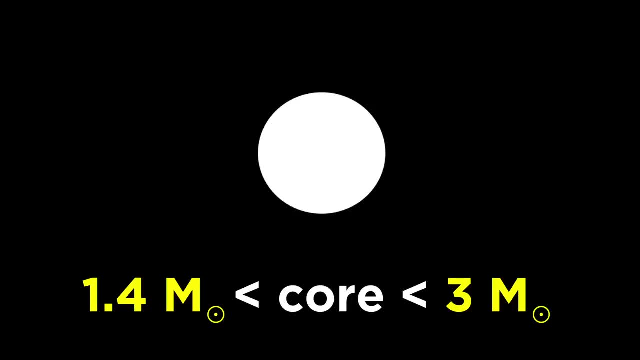 It's that 1.4 and 3 solar masses having been generated by a star that was originally somewhere in the ballpark of 10 to 40 solar masses, The core will not be able to support itself against gravity and it will collapse with. 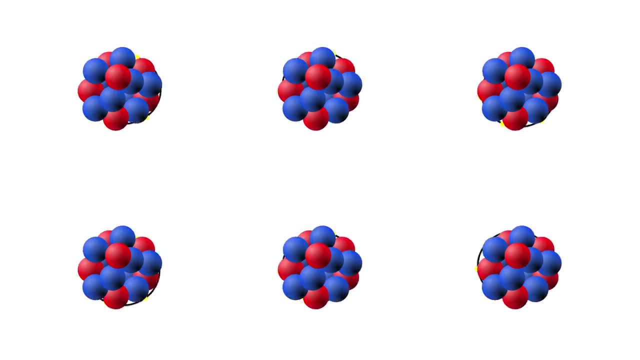 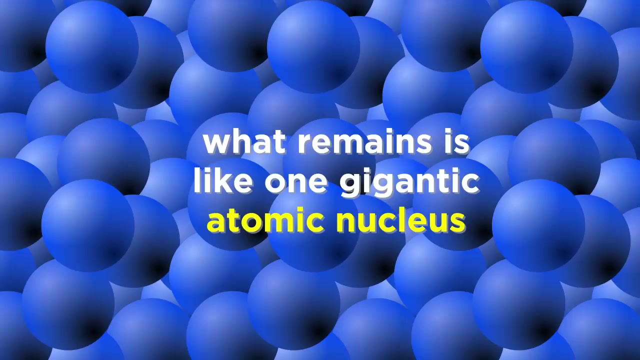 such tremendous force that all the electrons get squeezed into protons, such that they combine to form neutrons, and the shockwave from this event is what triggers the supernova. The object that remains is a ball of neutrons bunched up together like one huge atomic. 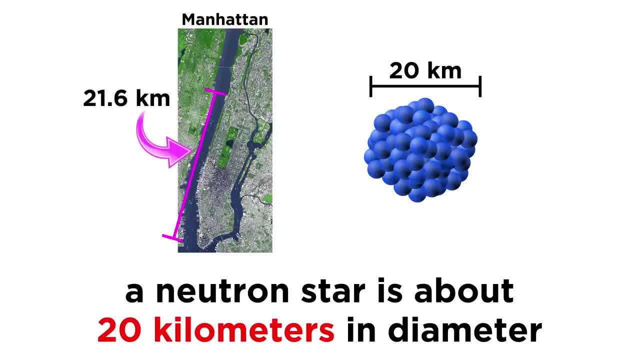 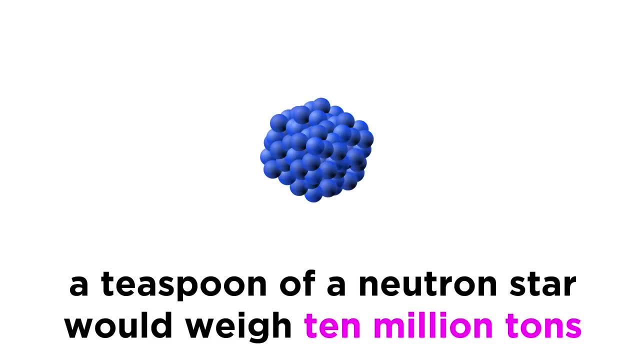 nucleus the size of New York City containing all of the mass originally within the core of the star. A teaspoon of a neutron star would weigh a whopping 10 million tons. But even more miraculously, if the core of the star is above around 3 solar masses even. 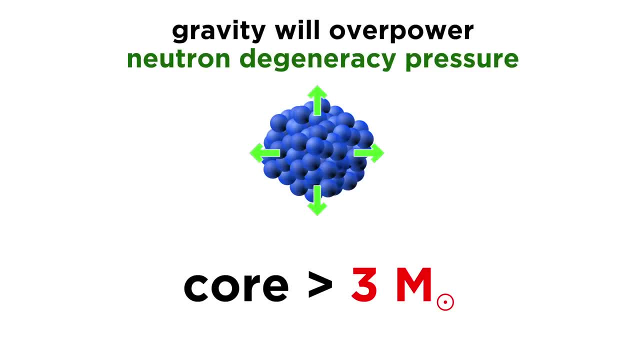 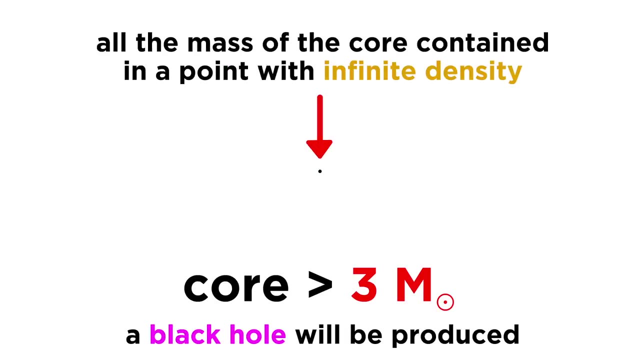 the outward mass of the star is less than 10 million tons. The outward pressure of neutrons pressing right up against each other, or neutron degeneracy pressure, is not enough to stop the immense gravity, and the neutrons will be crushed together as the remaining mass collapses into a single point of infinite density. 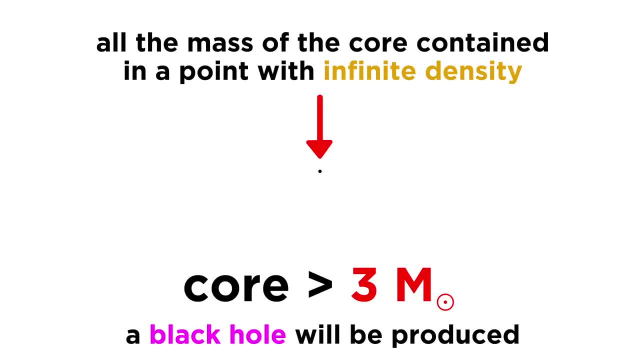 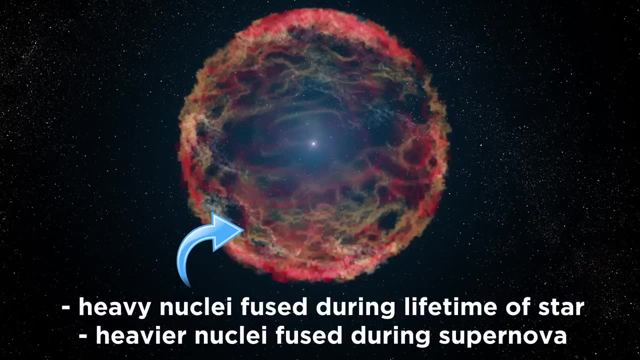 The entire mass of the star's core contained within zero volume. This object is called a black hole: The outer layers of the star that have been ejected full of heavy nuclei fused during the lifetime of the star, and the additional, even heavier ones formed during the supernova. 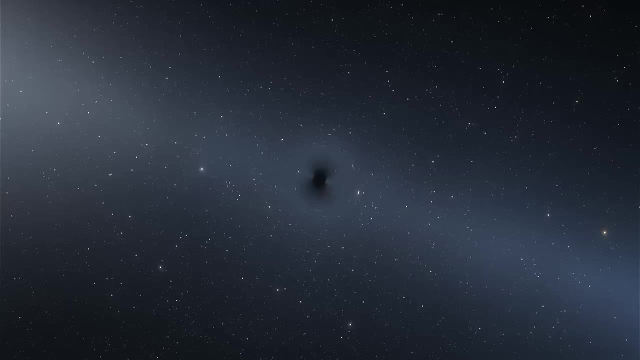 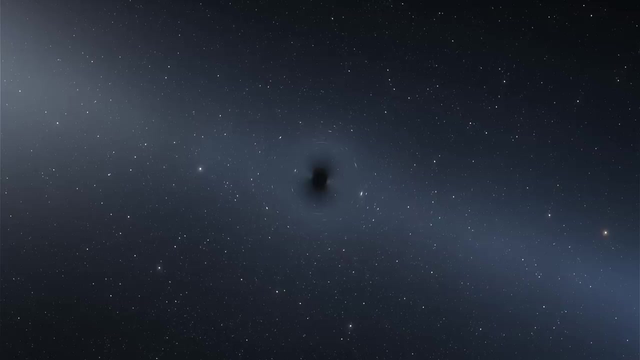 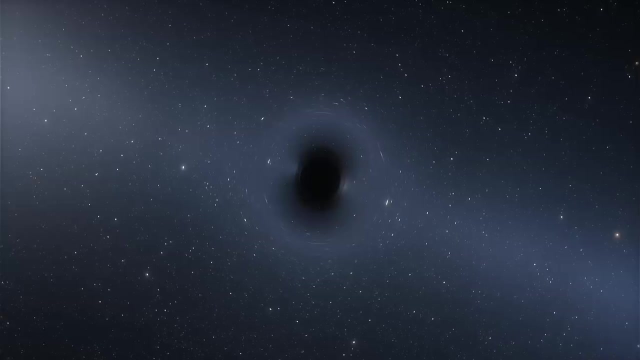 will leave behind a colorful nebula, But the singularity that is left behind is anything but colorful: A black hole, given its infinite density, warps spacetime so much that not even light can escape. Whatever a black hole might look like, if that can even mean anything, it's not a black hole. 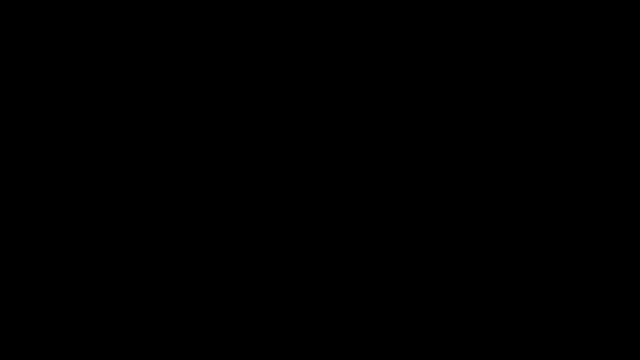 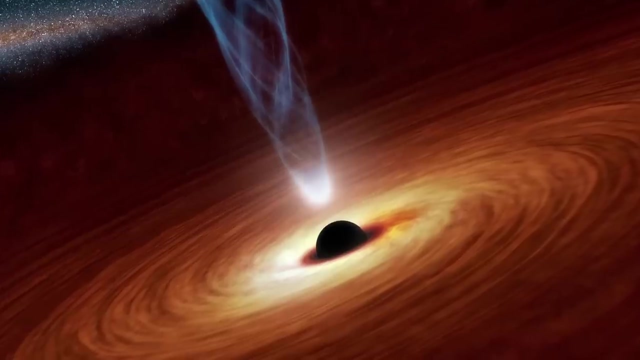 If it can even mean anything, we will probably never find out, because it is impossible for photons to leave it and reach our eyes, which is how we see things. As incredible as this may sound, this is how nature works, and black holes do indeed exist.